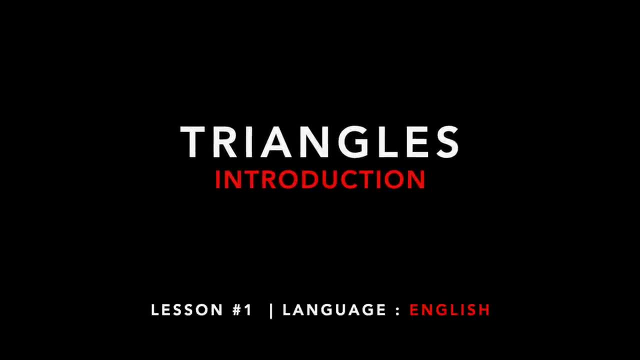 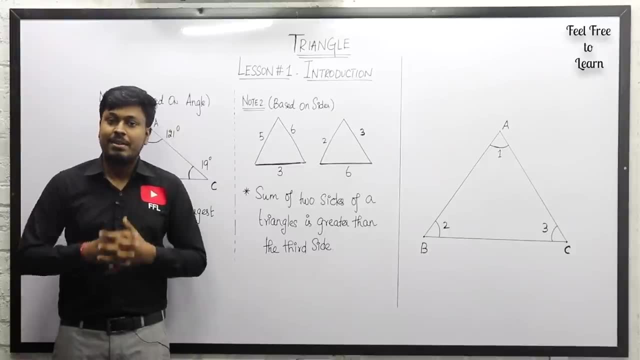 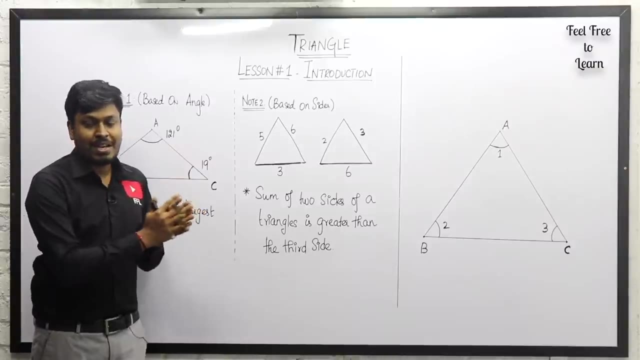 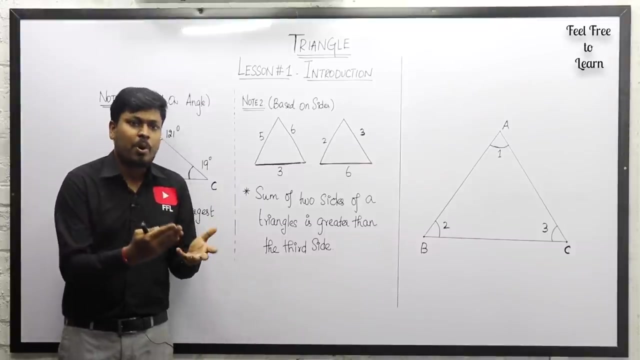 First of all, thanks for being here in my YouTube channel In this lesson number one on the topic triangle. So now I'm going to teach you the overview and introduction about this topic. So see here, triangle is one of the vast topic right where you have many properties and many 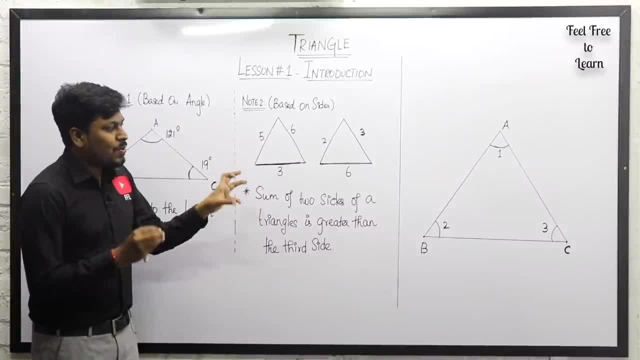 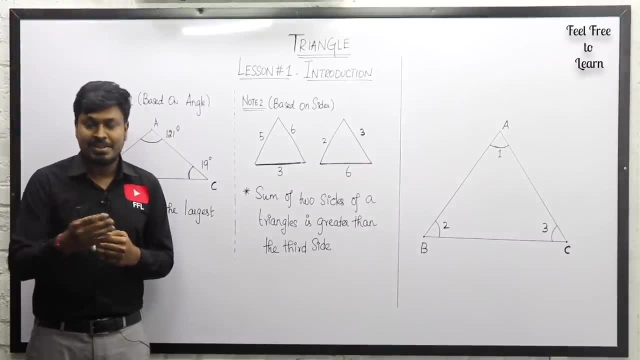 concepts. But in this introduction video I can teach you only the important concepts on the topic triangle. On the further videos I can teach you the properties and some of the concepts there Understood. So in this video we are just going to learn only the important concepts and some of 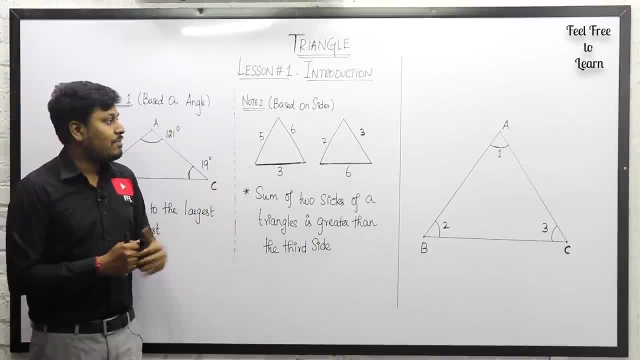 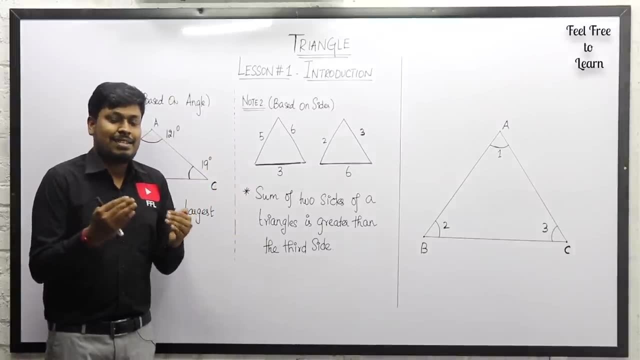 the important properties on the topic triangle. So now let me move on to this triangle topic. Just see what is a triangle. everyone knows that. we have learned in the schooling itself, right, What is triangle. Triangle is a plane figure which has three. 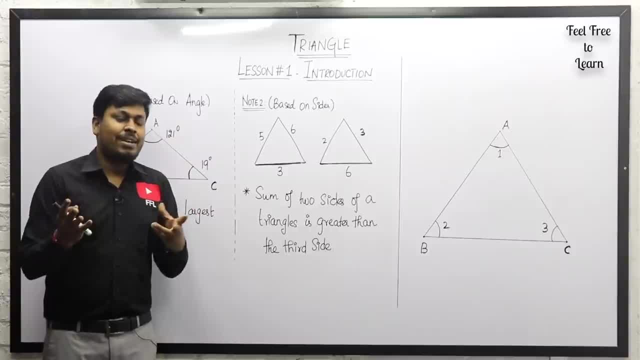 sides and three angles Understood, A plane figure is nothing but a two dimensional image. Triangle is a two dimensional image, right? So triangle is a plane figure or a two dimensional image which has three sides. See here: A and B will be side number one. B and C will be side. 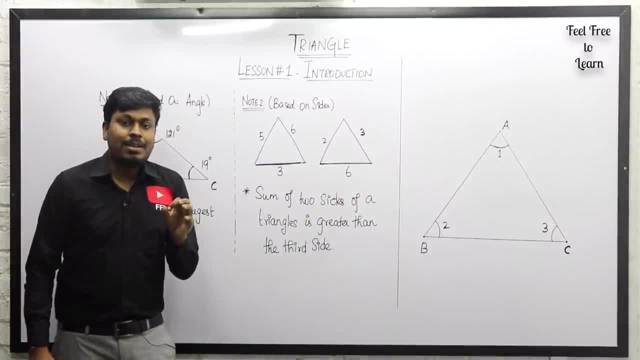 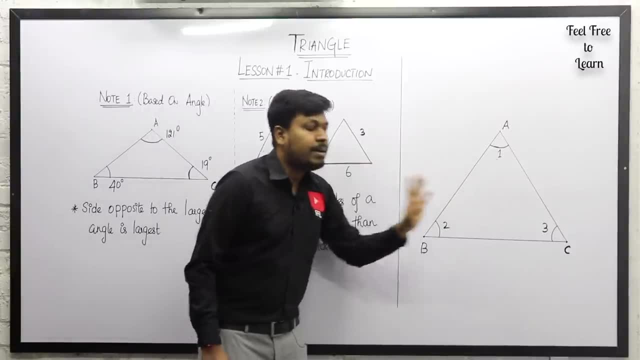 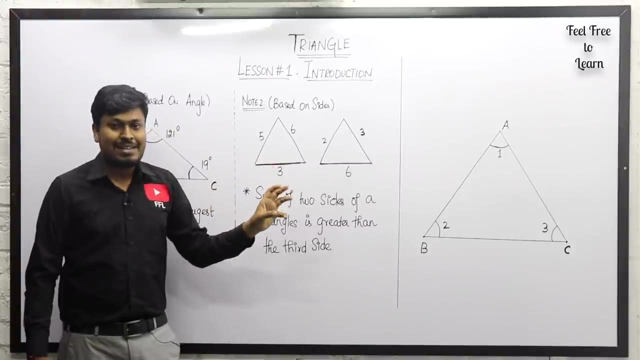 number two, C and A will be side number three. So totally a triangle has three sides And also it has three angles: right, So angle number one, angle number two and angle number three. So this is the definition of a triangle. So before solving some of the questions in a triangle, 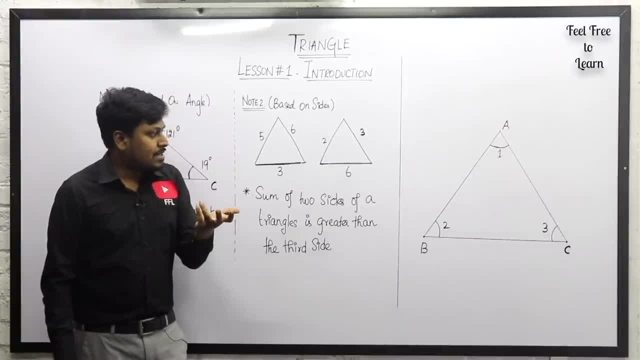 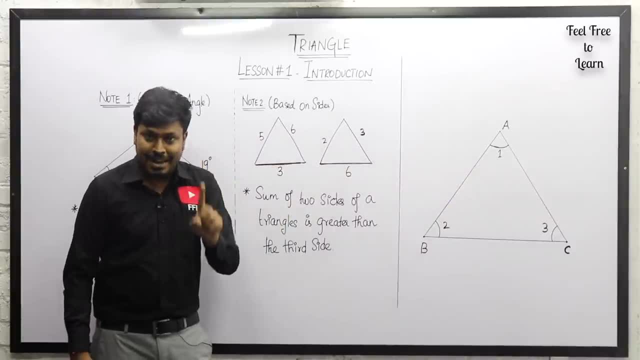 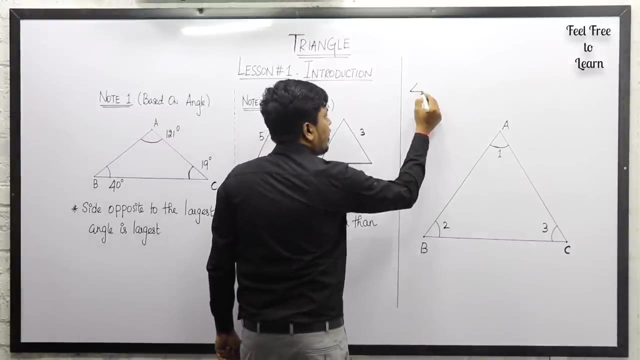 first you need to know some basic concepts, right? The thing is, if you add all the three angles- one, two and three, all the three angles of a triangle- it should always be 180 degree Understood. So always remember this point, most important point: If you add all the three angles, 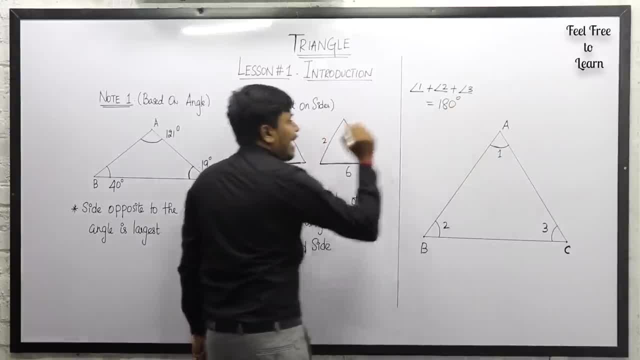 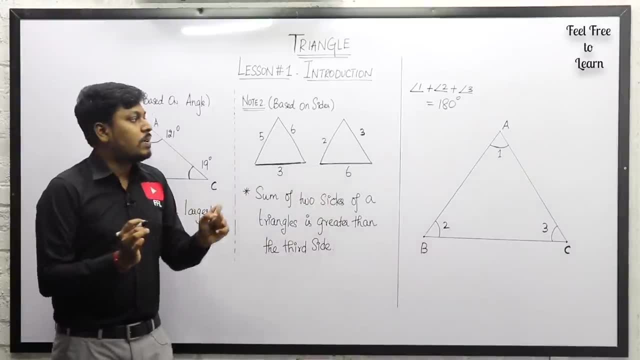 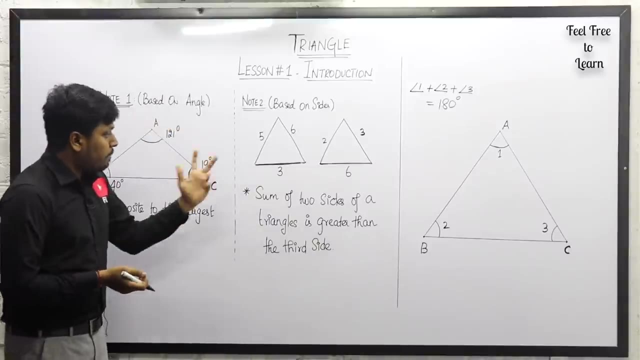 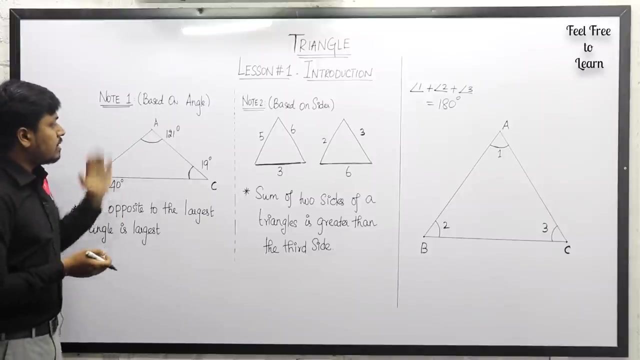 of a triangle, it should always be 180 degree. So this is the definition of a triangle. So this is the basic note on the triangle. So now let me move on to the two important notes here. One note is based on a side and the second note is based on an angle. Just see here note number one I have 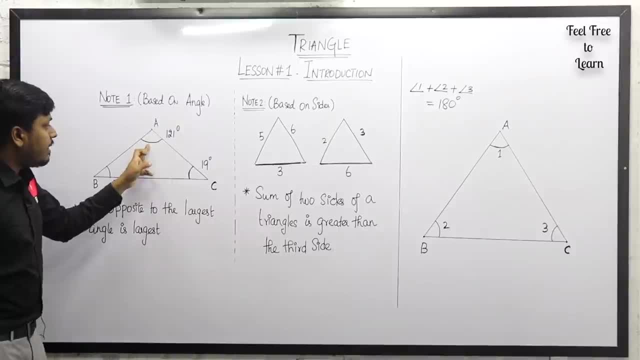 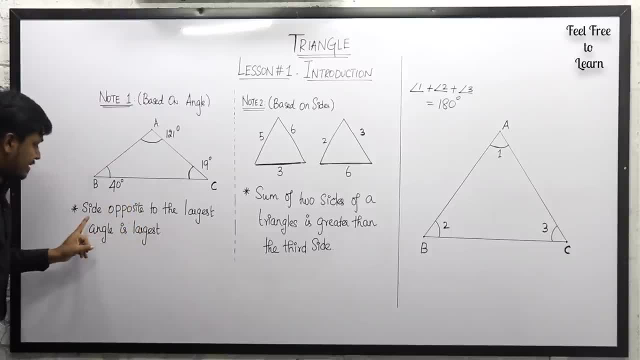 Angle C is 90 degree. Just look at this point carefully. Side opposite to the largest angle is the largest. So remember that the side opposite to the largest angle, here, in this three angle, which angle is largest? 121 degree is the largest angle. So the side right, this side which is 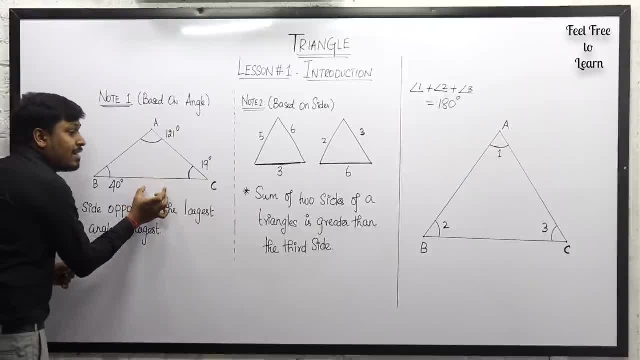 opposite to the largest angle is always largest, which means the distance between B and C will be higher. Friends, understood, Just see here: side opposite to the largest angle. So largest angle is 121 degree, which is A right So side. 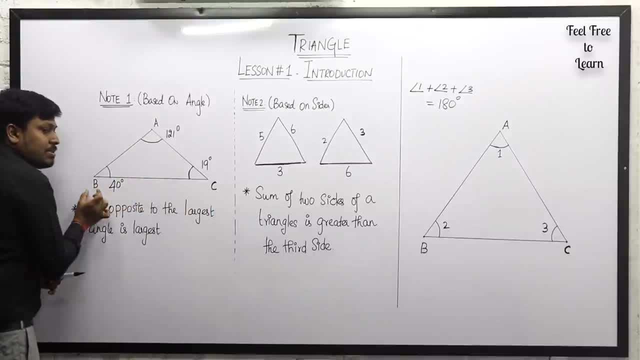 that is opposite to the largest angle, which is B and C. So this distance will always be largest when compared to other two distance. So, friends understood. So here, the distance B and C will always be largest when compared to other two sides Understood. So this is the point number. 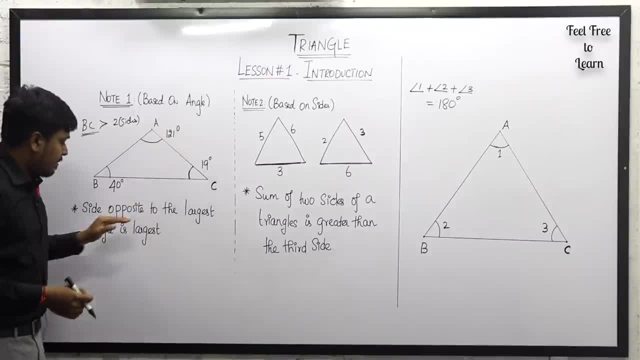 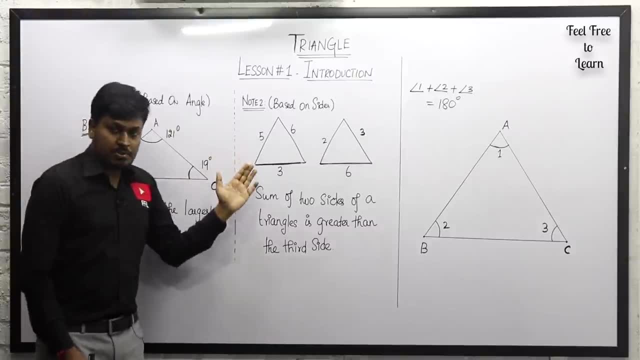 one that you need to know that is based on an angles. So remember the distance between B and C will always be largest when compared to other two sides. So remember side that is opposite to the largest angle will always be largest. And note number two. So here it is based on the sides. 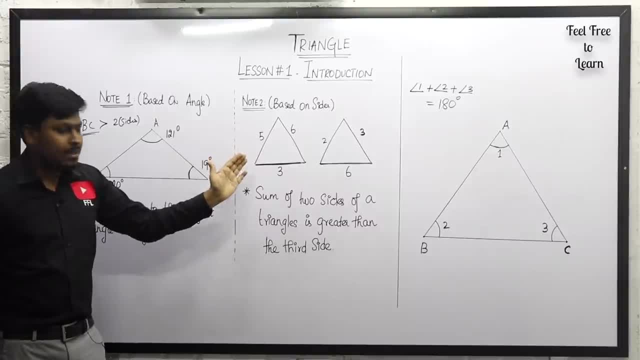 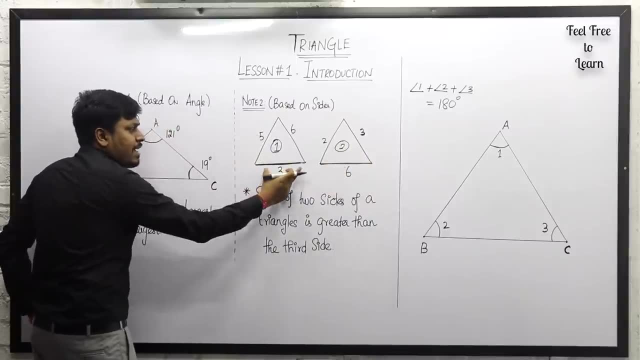 Just see, here I have drawn a two example triangles here, This first example triangle and this will be the second example. Just see the triangle sides of. assume that this side will be three centimeter and another side will be five centimeter and another side will be six centimeter. Just read: 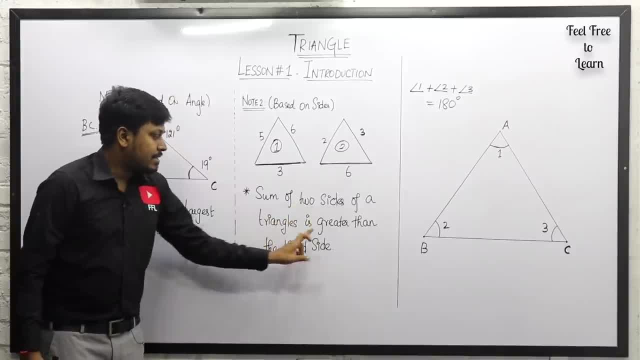 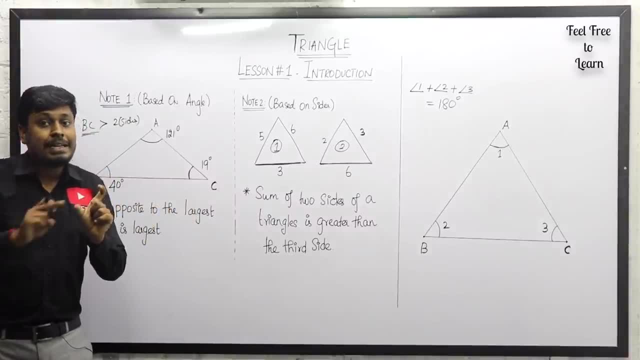 this note: Some of two sides of a triangle is greater than the other side. So here the distance between B and C is greater than the third side. So if you add two sides of a triangle it should always be greater than the third side. So let me take this example number one: Add any two sides of 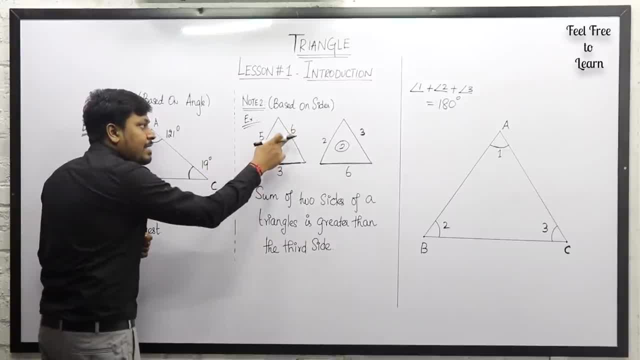 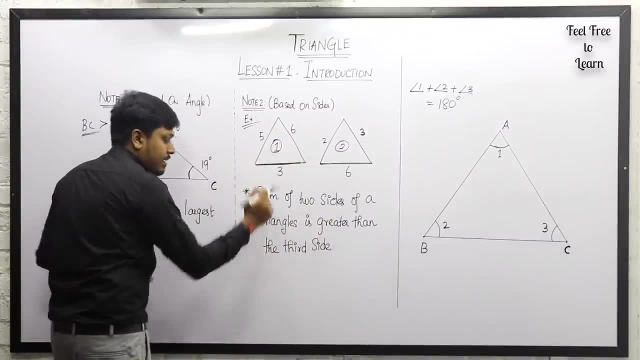 a triangle. I can add this: five plus three is eight. So eight is greater than six, or not? Yes, it is greater than see some of two sides of a triangle. I am just adding five and three here, So five plus three, which is eight. So some of two sides of a triangle is always greater. 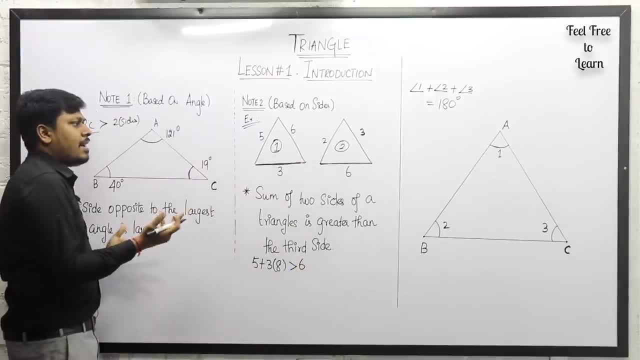 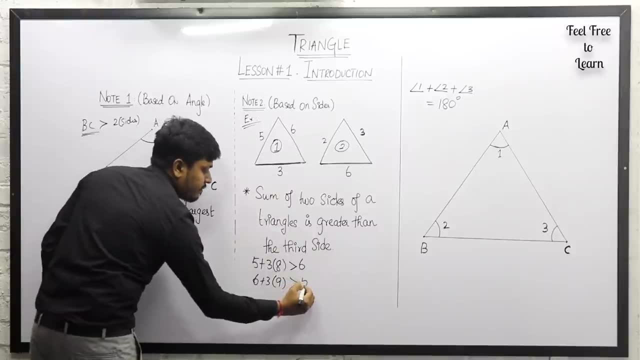 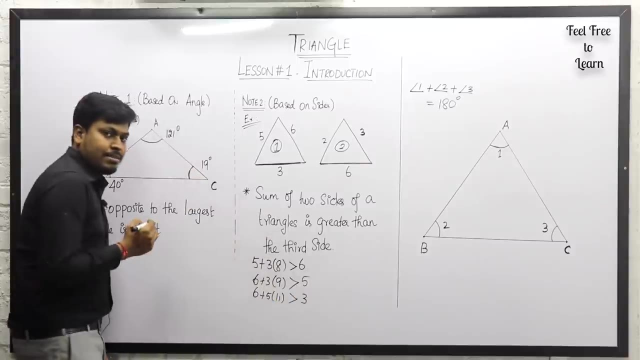 greater than the third side, Yes or no? Yes, it is greater. Add another, another, any two sides, just see six plus three. So six plus three will be nine. it is greater than the third side, which is five. Again six plus five, So which is 11?? It's again greater than three. Yes, So we can. 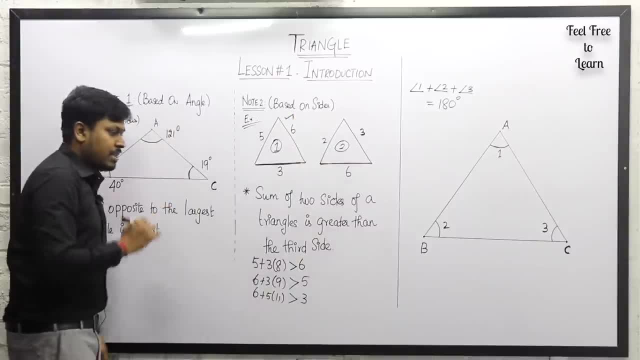 say it is a triangle. it satisfies the basic rule Understood Some of two sides of a triangle, any two sides. if you add any two sides of a triangle, it should be greater than the third side. So we can say this example number one is satisfied, So we can say it's a triangle. 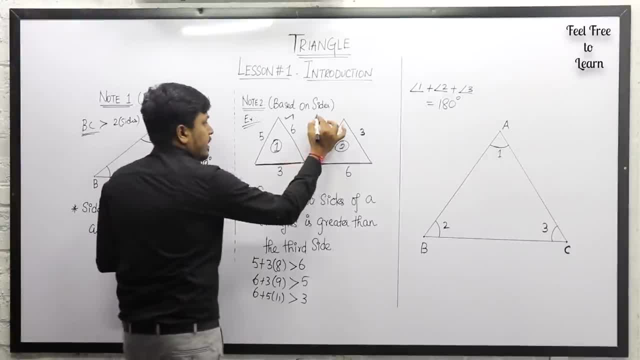 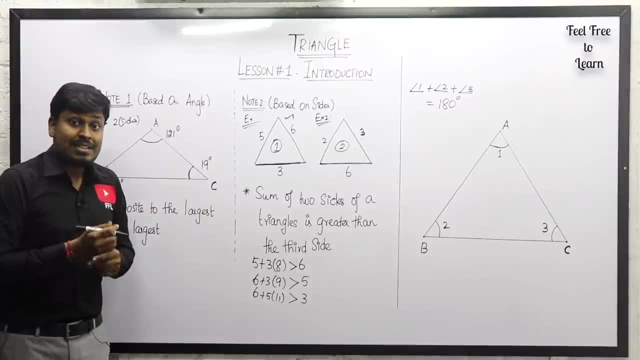 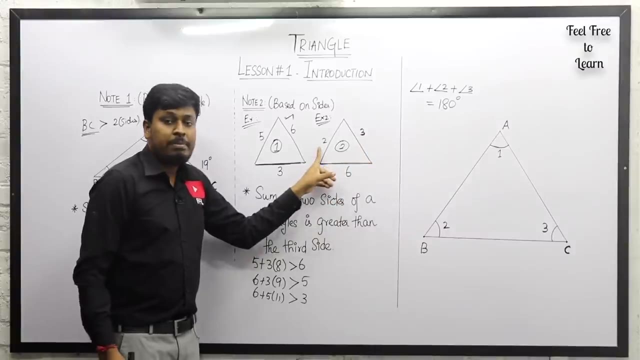 Let me move on to the second example, right, So example number two here. Just check whether this diagram is an exact triangle or not. Add any two value and check whether it is greater than the third side. So if I add three and two, just see three plus two will. 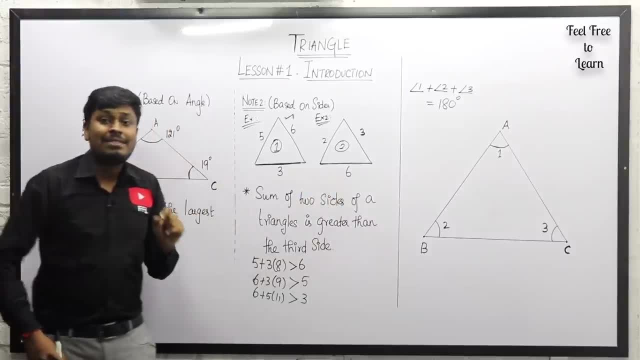 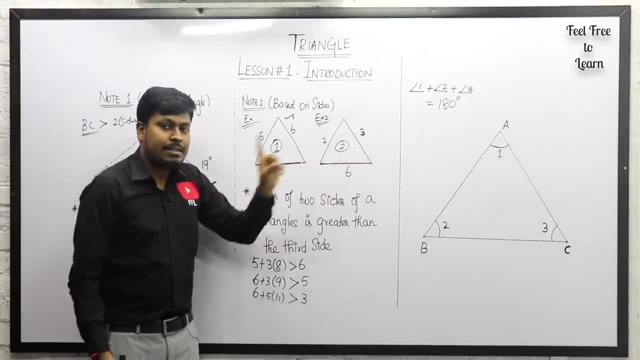 be five. Whether five is greater than six, No five is lesser than six. Understood, If I add six plus two: yes, six plus two is eight, So eight is greater than three. Add another side: Six plus three is nine. Nine is greater than two. Yes, satisfied. But when you add these two sides, 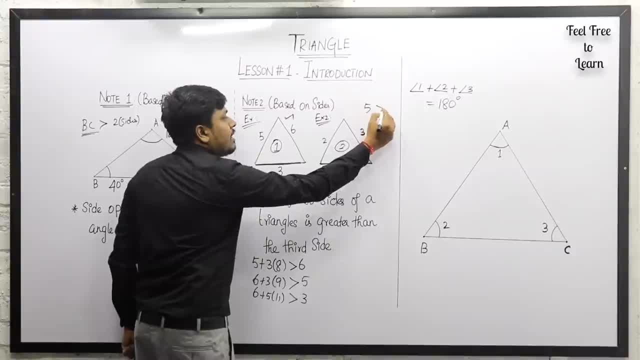 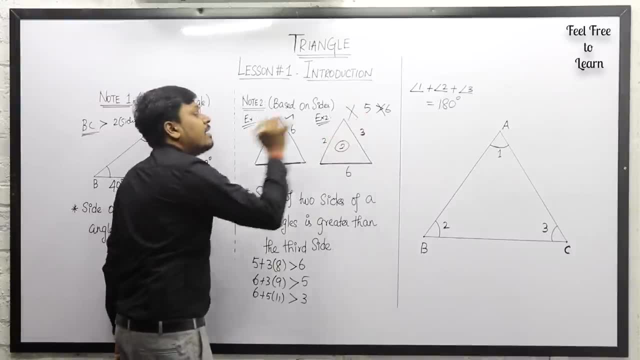 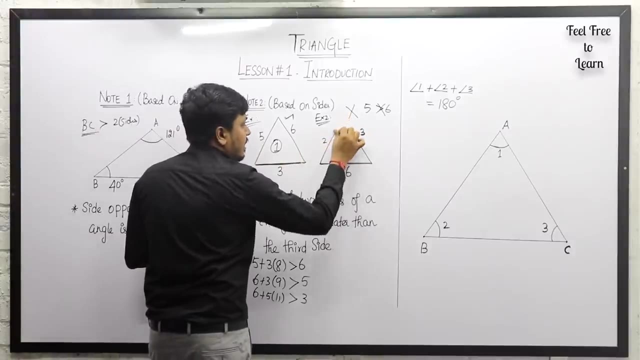 three plus two is five. Five is not greater than six. It is definitely lesser. So it does not satisfy the basic rule. So it is not a triangle. If you draw the diagram perfectly how this triangle looks like, Just see here the triangle will be exactly looking like this. So it is not. 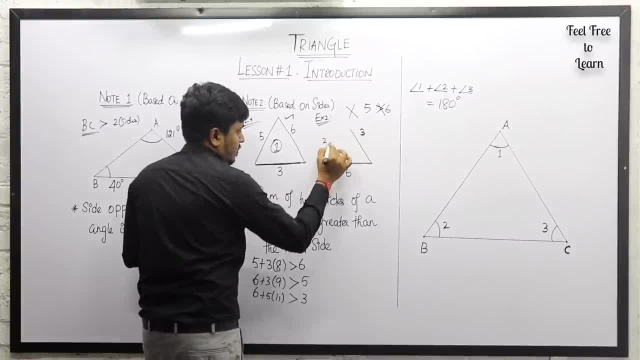 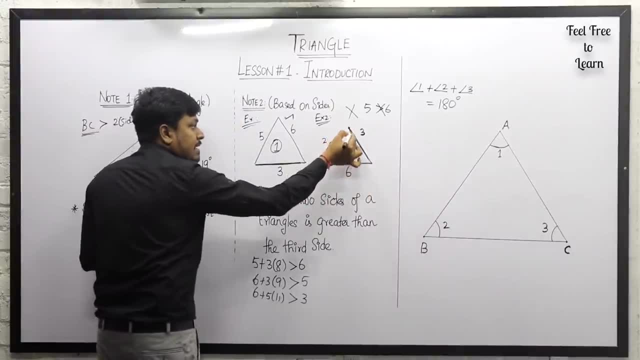 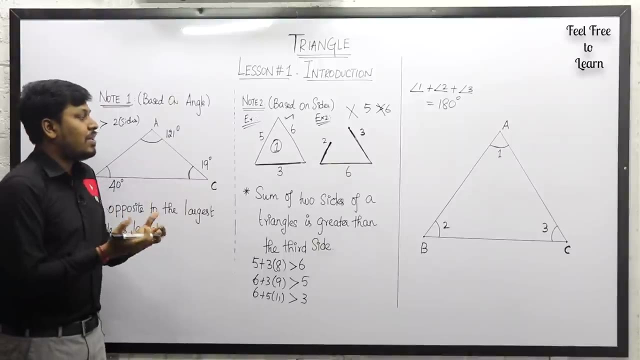 like this Understood, Because we know that this is six centimeter and this is three centimeter and this is only two centimeter. So definitely it is not a triangle, Yes or no, right? So we can surely say that example number one is a triangle, but example number two is not a triangle because it. 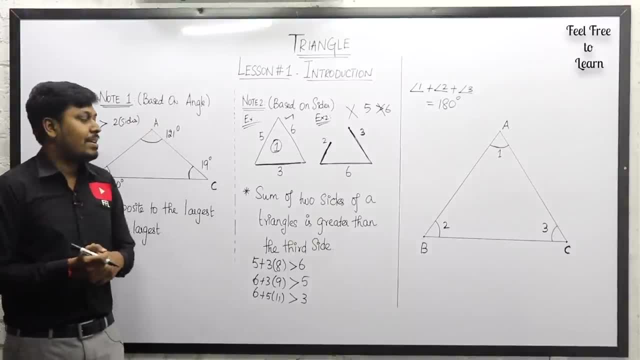 does not satisfy the basic rule itself. So we can say: example two is not a triangle. So, friends, these are the just simple thing that you need to know before solving a question. There are different types of triangles and different types of note, But these two are the most. 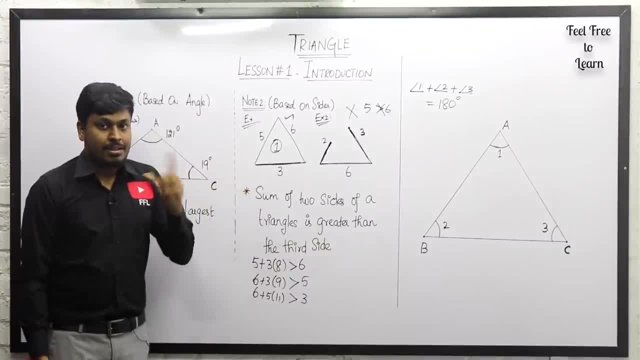 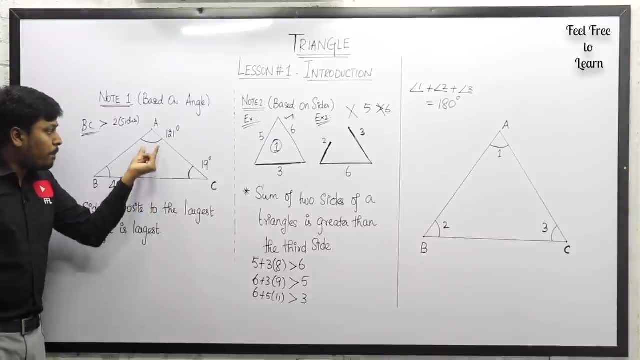 important note if you need to solve some of the basic questions. The first note, which is based on an angle. So what I have said here is side that is opposite. So the side which is opposite to the largest angle will always be largest. So the distance between B and C, the length, will be. 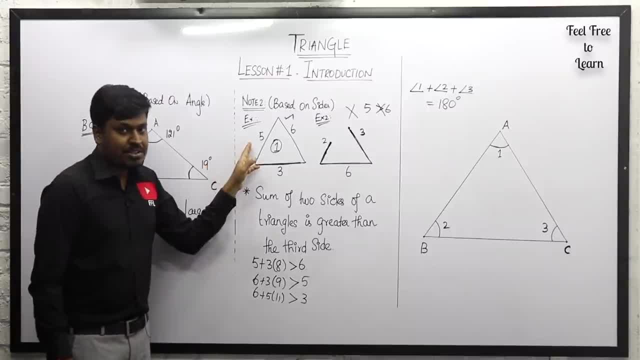 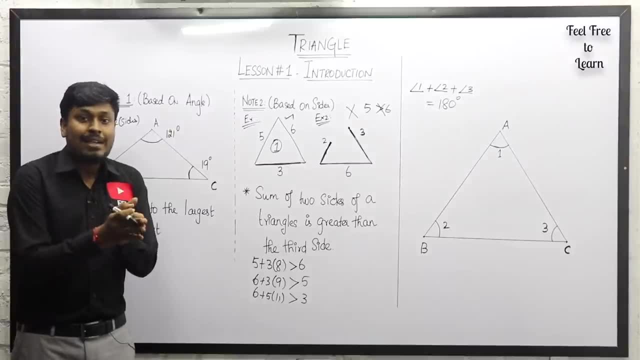 always largest Understood. So point number two, that is, B and C, is based on side. If you add any two sides of a triangle it should always be greater than the third side. If it is not greater than the third side, then definitely it is not a. 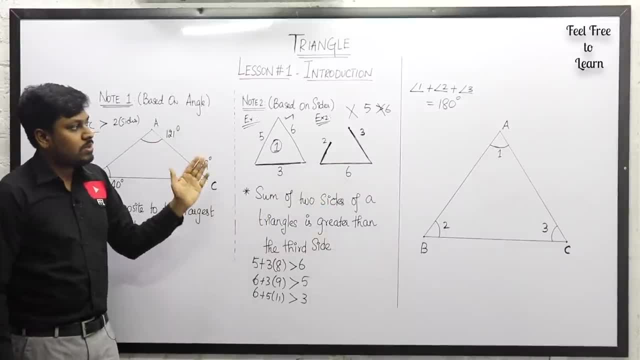 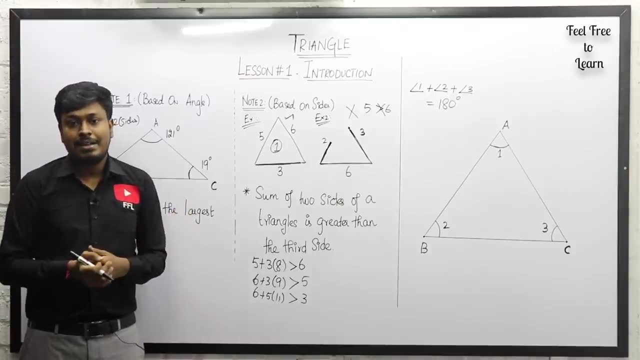 triangle Understood. So these are the two important notes in the topic triangle. So now let me move on to some of the types of triangles. what are all the different types of triangles are there, And also we can see what is acute angle, what is obtuse angle, etc. So now we can see what are all. 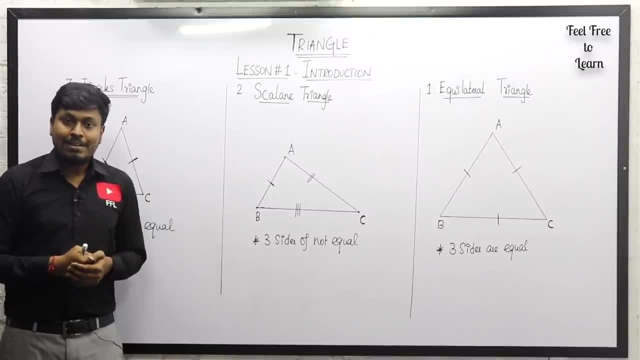 the different types of triangles are there. So, So totally. there are three different types of triangle, and the first one is equilateral triangle, and the second one is scalant triangle and the third is isosceles triangle. So let me move on to the first type of triangle, that is, equilateral triangle, In the word itself, where you can find the word equi, which is equal. 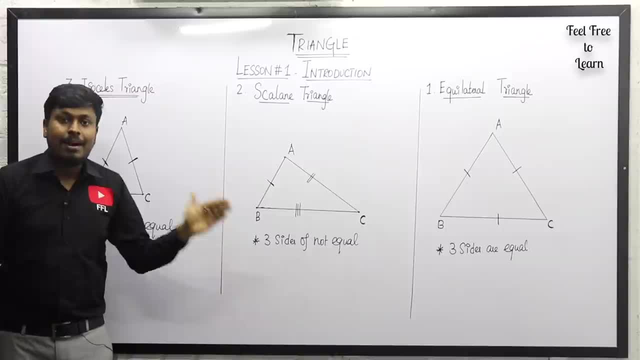 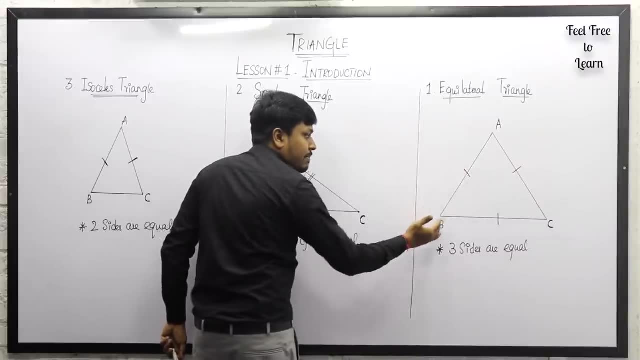 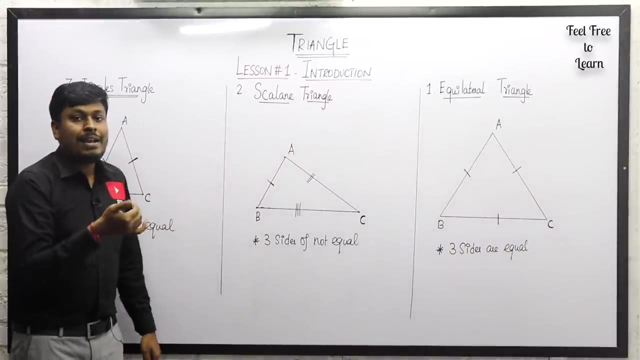 So if all the three sides of a triangle are equal, then it is called as equilateral triangle. Understood, Just see here. So AB will be side number one, BC and AC, So all the three sides are of equal in length, then it is called as equilateral triangle. 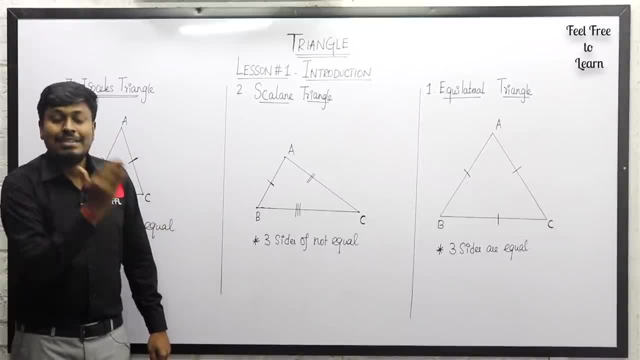 So if all the three sides of a triangle is equal, then it is called as an equilateral triangle, Understood, If all the three sides are equal, then the angles are always be equal, because if sides are equal, then all the three angles will also be equal. 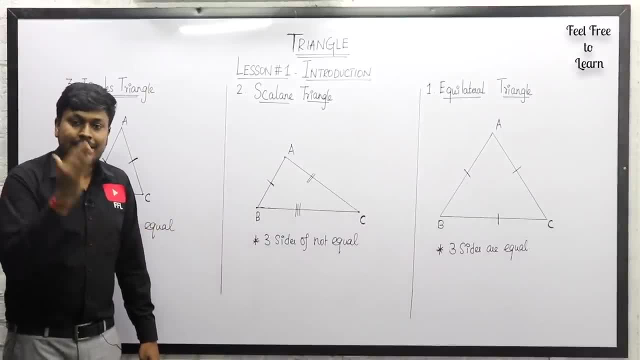 So friends understood. So if it is an equilateral triangle, three sides will be equal. So three angles also be equal, Understood. So second triangle is a scalant triangle. So here all the three sides of a triangle are not equal. 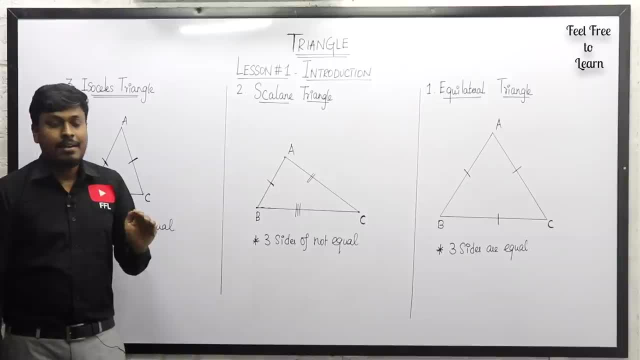 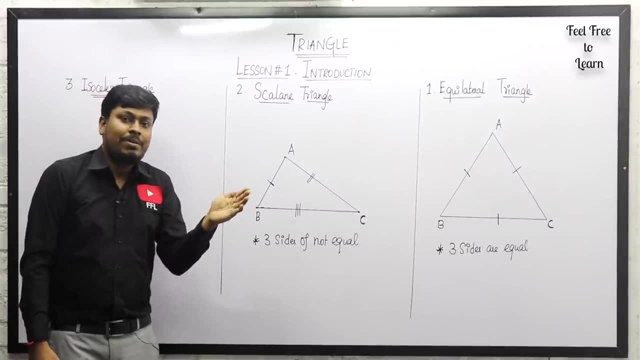 Understood, Which is called as an scalant triangle. If all the three sides are not equal, then the angle will always be not equal, Because if sides are not equal, then angle will be different. right? So if it is a scalant triangle, what is the meaning of scalant triangle? 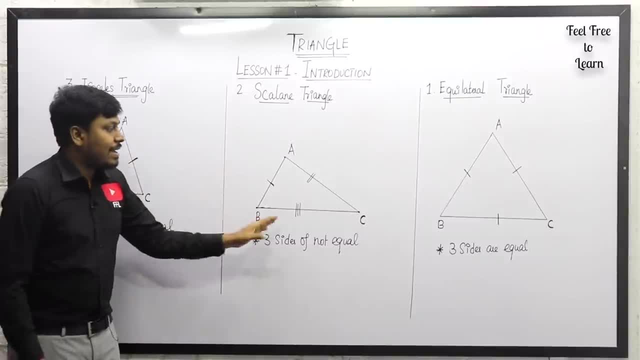 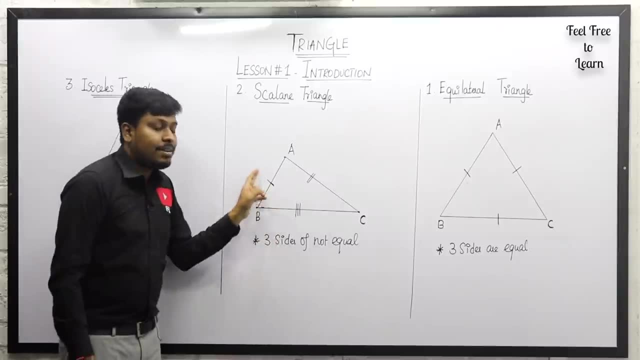 What is the meaning of scale and triangle? All the three sides of a triangle is not equal, which as different in length? and another important point is: if all the three sides are not equal, then the angle will also be not equal. Got it? All the three angles will also be different. 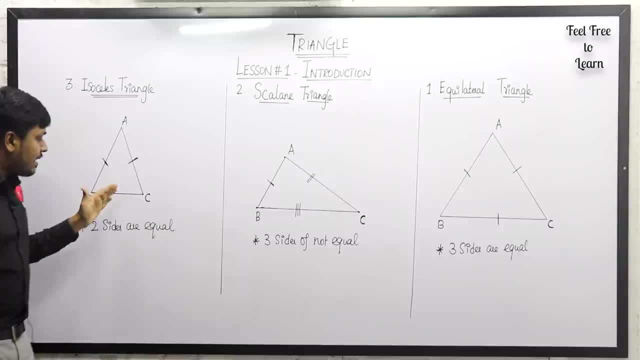 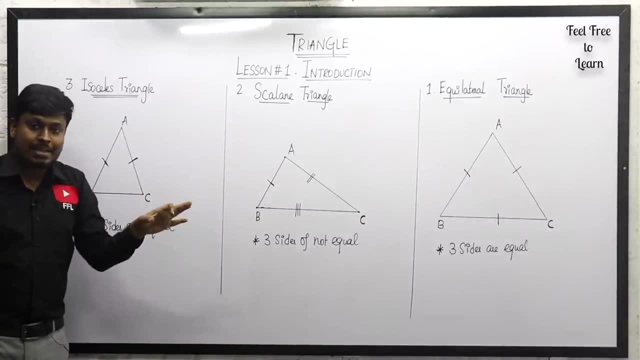 So the last is an isosceles triangle. So if it is an isosceles triangle, two sides will be equal. If it is an equilateral triangle, all the three sides are equal, but if it is an isosceles triangle, only two sides will be equal. So if two sides are equal, then we can say that two angles will be equal. Out of three, two angles will be equal. 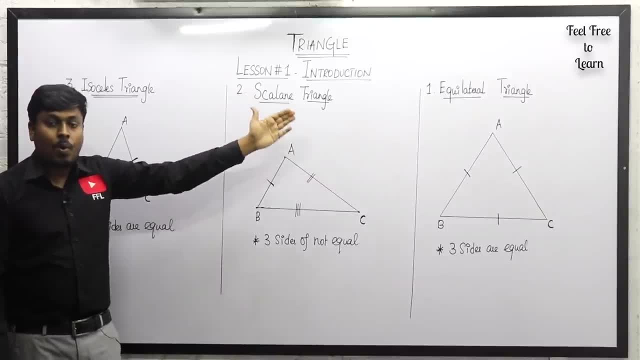 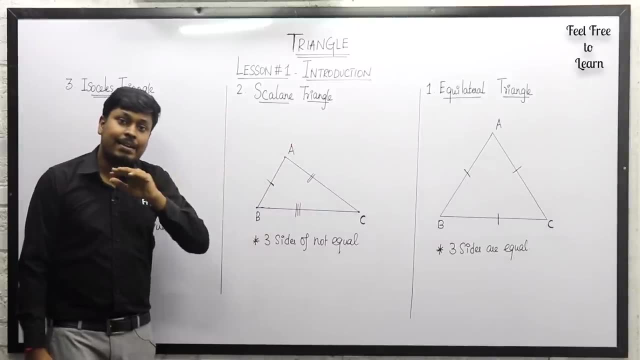 Understood, friends Right. So if it is an equilateral triangle, all the three sides of a triangle are equal. If it is a scale and triangle, all the three sides of a triangle are different in length. If it is an isosceles triangle, only two sides will be equal in length. 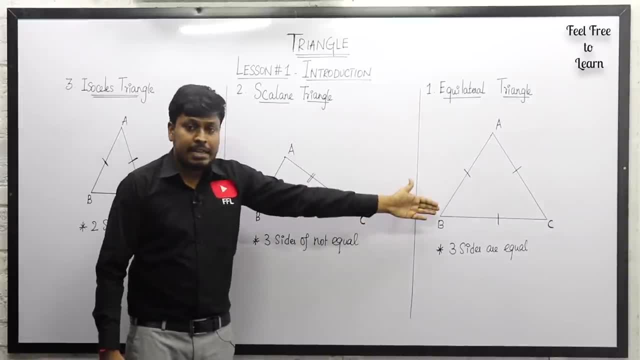 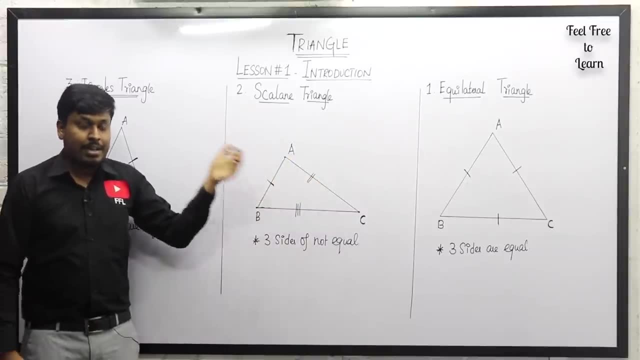 And remember, if it is based on angles, if it is an equilateral triangle, all the three angles will be same. If it is a scalar triangle, all the three angles will be different. If it is an isosceles triangle out of three, two angles will be same. 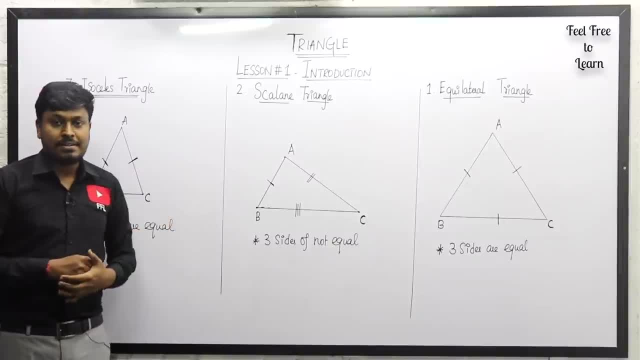 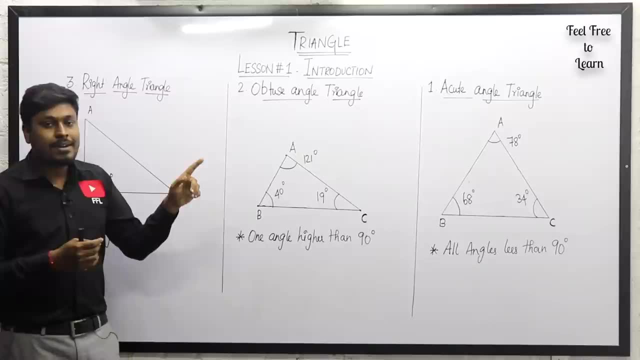 Understood. So this is the different types of triangles. So now we can see the different types of triangle that is based on angles. So number one is acute angle triangle, number two is obtuse angle triangle and number three is right angle triangle. 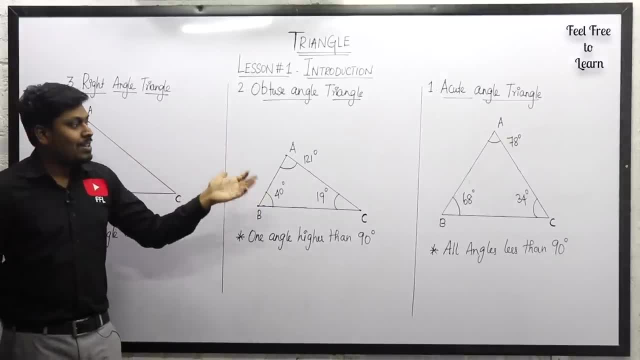 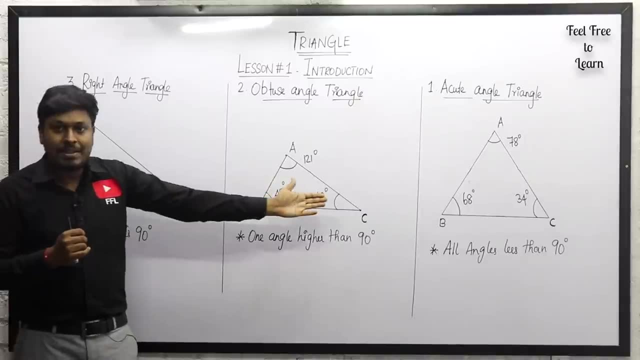 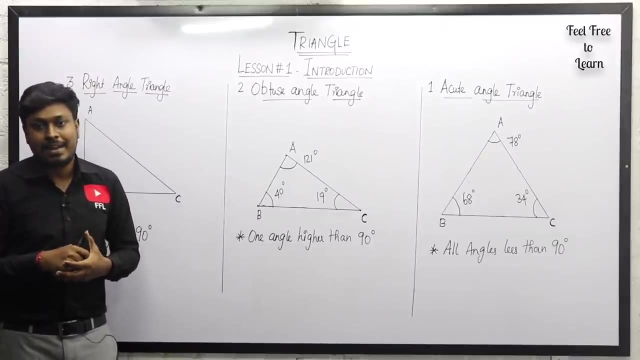 I think all these steps we have learnt in the schooling itself. So let me move on to the first type, acute angle triangle. So acute angle triangle is in this triangle, in the given triangle. if all the three angles are length less than 90 degree, then it is called as an acute angle triangle. 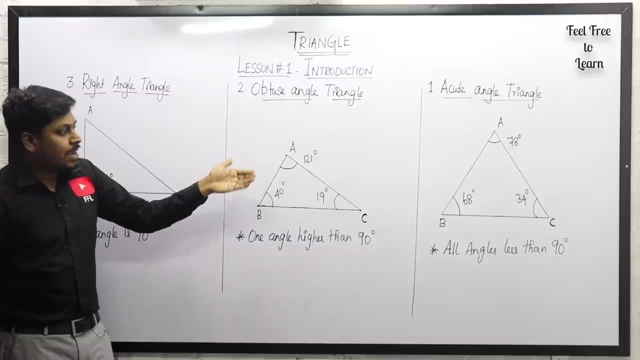 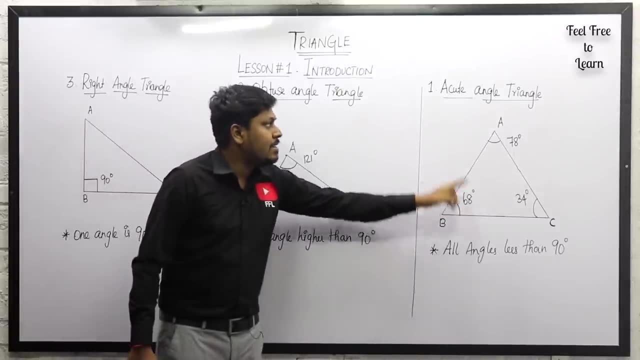 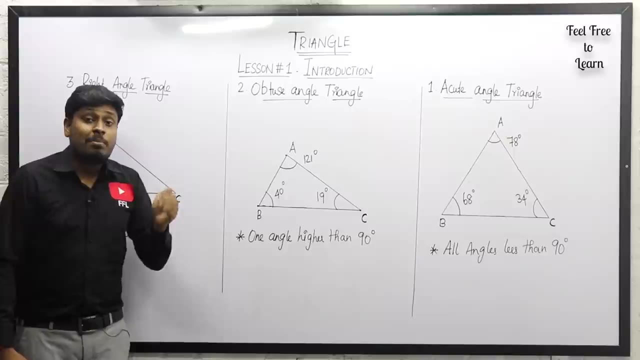 Just see, the first angle is 78 degree and the second is 68 and the third is 34.. So all the three angles are less than 90 degree. So we call this triangle as acute angle triangle, In case, if any one angle, any one right, if any one angle is more than 90 degree, then it is called as an obtuse angle triangle. 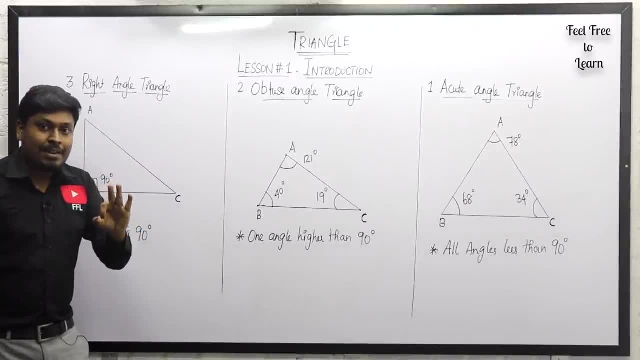 Got it In case out of three angles. if any one angle is exactly 90 degree, then it is called as a right angle triangle. I hope everyone knows this, But sometimes there might be students who forgot what is called as acute and obtuse.